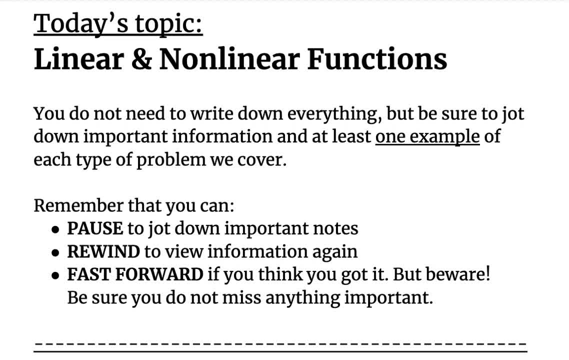 Hi everyone. today we're talking about linear and nonlinear functions. As a reminder, you do not need to write down everything that we'll cover in this video, but be sure to jot down important information and at least one example of each type of problem that we'll cover. Also, remember that you can pause to jot. 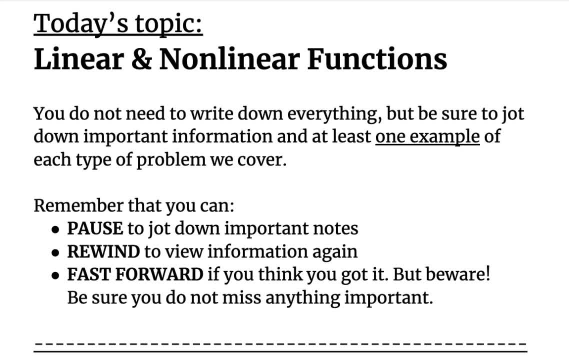 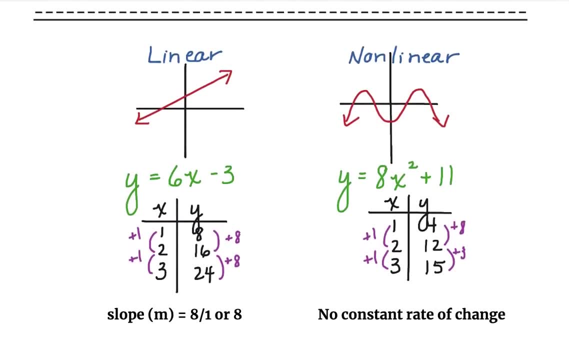 down important notes, rewind to view information again and fast-forward if you think you already got it. Just be careful make sure you don't fast-forward too much, that you end up missing out on something important. So functions can either be linear or nonlinear. So here are two examples. A linear function: 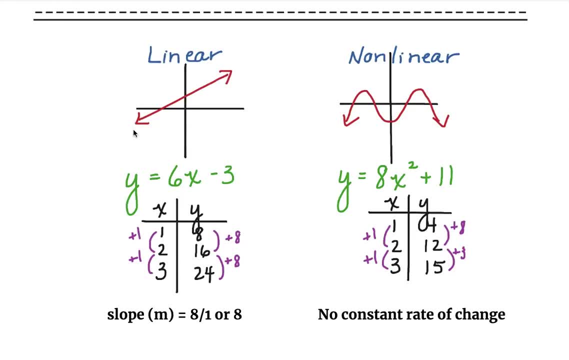 as you can tell, makes a straight line for the graph. A nonlinear function does not make a completely straight line on the graph. They could also give you a table of the values and that's like the XY points without the graph. So we're. 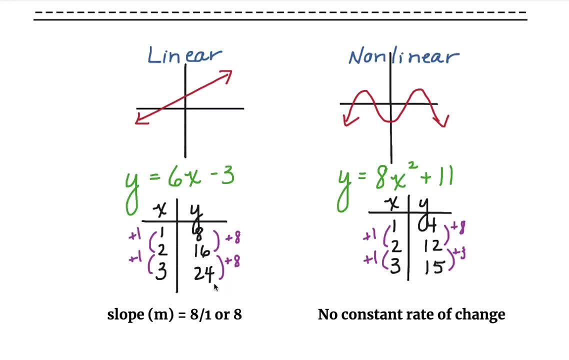 gonna go over that as well. If you're just given the table of values, the XY values from your ordered pairs, you will need to calculate the slope and the slope will let you know if it is linear or nonlinear. So if you remember calculating slope, you are subtracting. 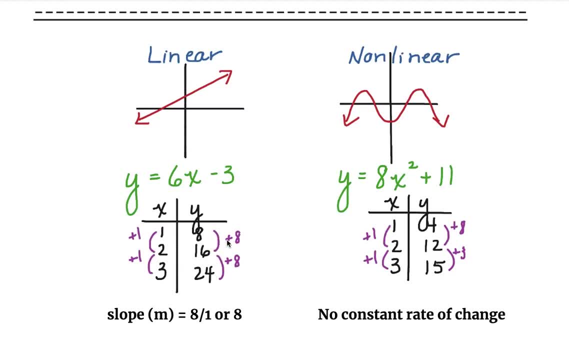 the Y's and you're subtracting the X's and then you are dividing them. So change of Y over change of X. So here the Y's are going up by 8 each time and the X's are going up by 1's each time. 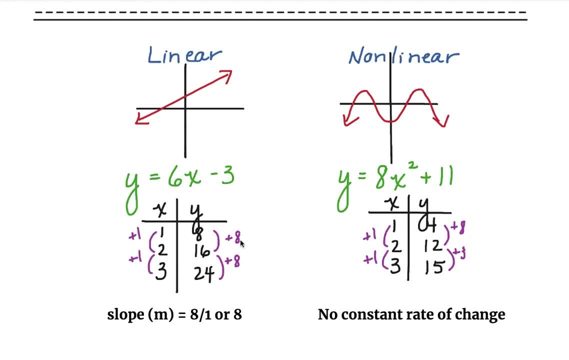 That's the difference between the Y values. So the differences of Y's is on top, 8 over your differences of X, which is 1.. 8 divided by 1 is 8.. So we know it's going to be a straight line, because it's always 8 over 1.. 8 over 1 each time you look at the values. 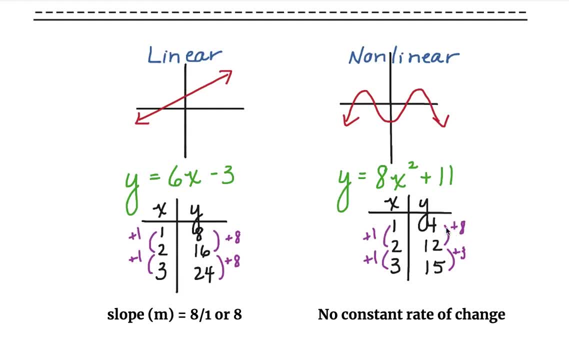 For a nonlinear function, the slope or rate of change is not the same. So on one hand I have 8. over 1 for two different pairs of points and on the other hand I have 3 over 1 or 3 for two other points. So it's not a constant rate of change. Sometimes it's. 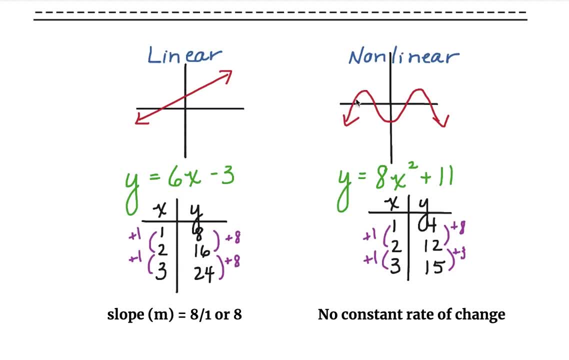 going up by 8 like really fast, and other times it's going up by 3 really slowly and I imagine for this line it's going to go negative as well for other parts. The other thing you probably notice is that the equations look different Linear. 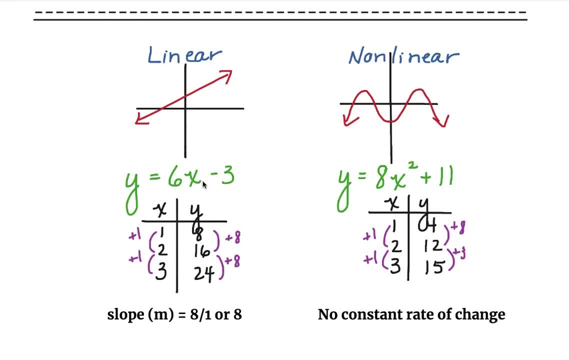 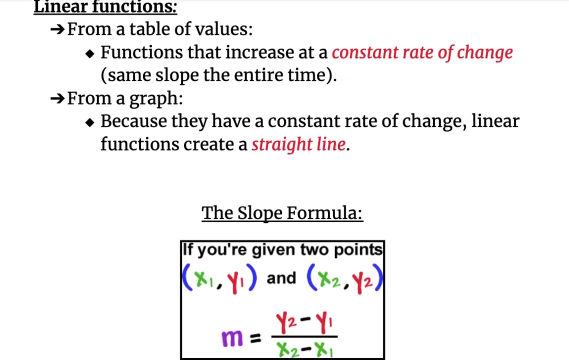 functions always have just x to the first power, a normal x and nonlinear functions are going to probably have x to a different power or exponent. Make sure you jot this down before we move on. So, as a review, linear functions from a table of values you can find them. find. 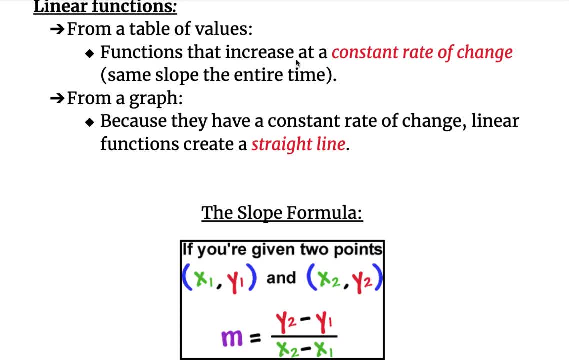 out whether it's linear or linear functions from a table of values. you can find them, But find out whether it's linear or linear functions from a table of values. you can find them, but find out whether it's linear or not, because functions that increase at a constant rate of change. so 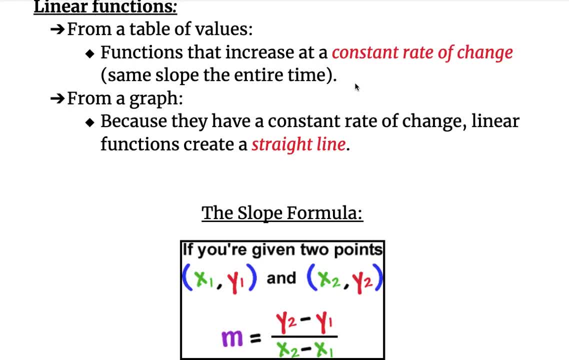 same slope the entire time are going to be linear. To figure out if it's a linear function from a graph, it's going to create a straight line and that's because they have a constant rate of change. And, as a review, here is the slope. 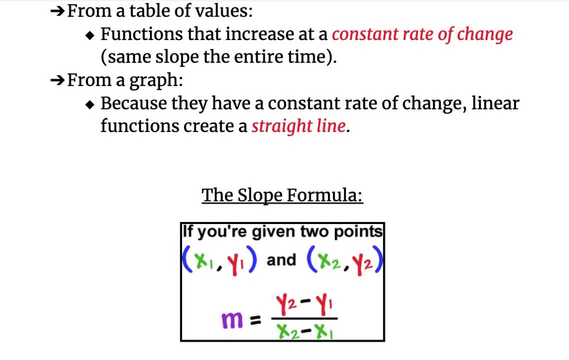 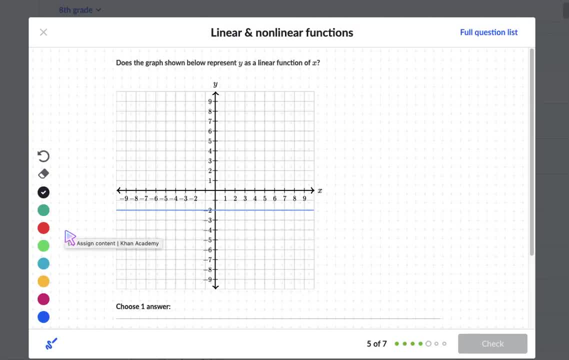 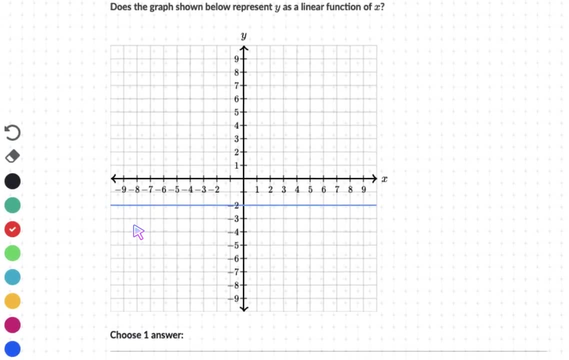 formula again. So again, pause the video and make sure you have this in your notes. All right, let's move over to some examples, so that we can practice what we just talked about In this problem. they want you to know, want you to figure out. 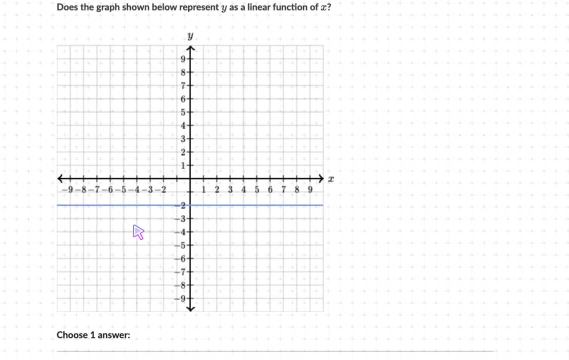 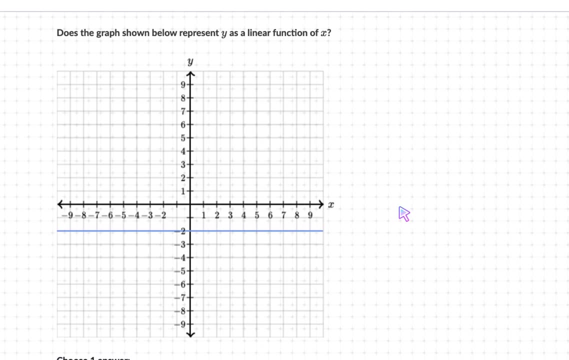 does the graph shown below represent y as a linear function of x? So it's just either a yes or a no. Go ahead and pause the video and try it on your own first. All right, so I see a straight line and I'm going to make sure that I have a. 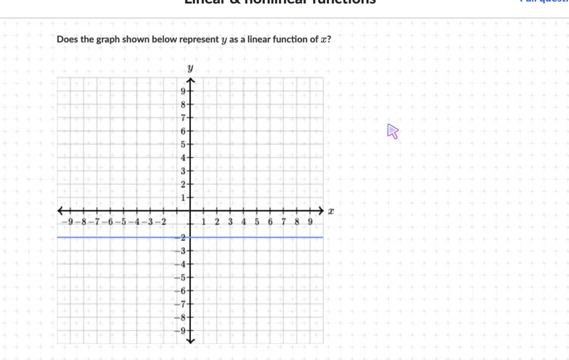 straight line going across. it is completely straight. So I'm going to assume that it is, yes, a linear function. The other way I could check- and this is totally not necessary- is I can create an x- y table. So I'm going to figure out. 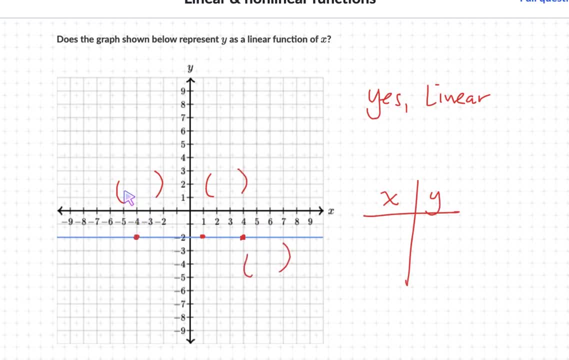 the ordered pairs and just the three points is fine. This is negative, four negative five, two. this is one negative two and this is four negative two. So my x- y's are negative, four negative two, one negative two and four negative two. That's how we create the table of values. 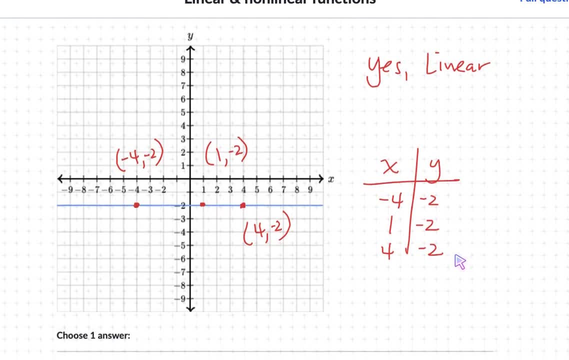 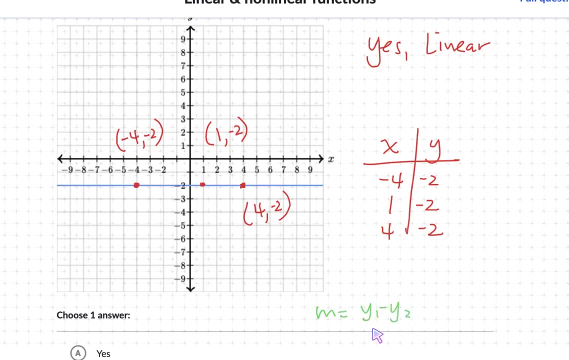 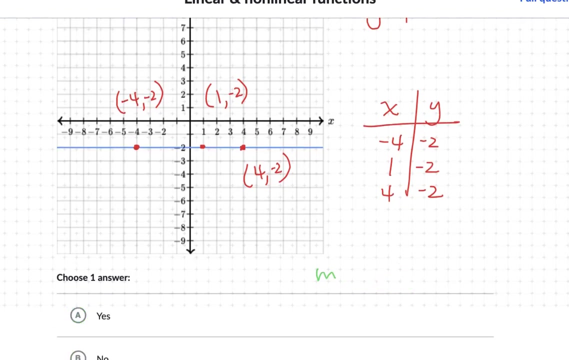 And remember, we have to figure out the slope. Slope is the change of y over the change of x. So I'm going to subtract my y's on top and then I'm going to subtract my x's on the bottom And that's basically our rise over run From our table. we can just do an easy subtraction here. 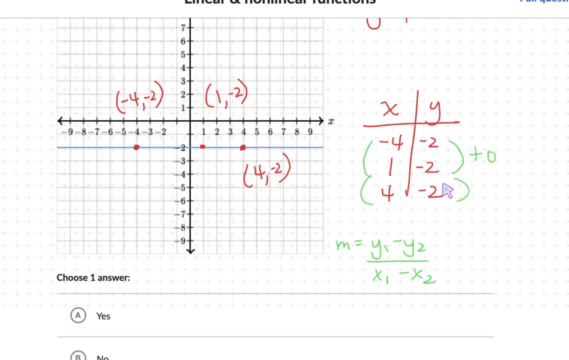 To get from negative two to negative two. I didn't do any changing. Negative two to negative two: also no changing. So I'm going to subtract my y's on top and then I'm going to subtract my x's on the bottom. Negative four to one, let's see. I would add five to get there And then 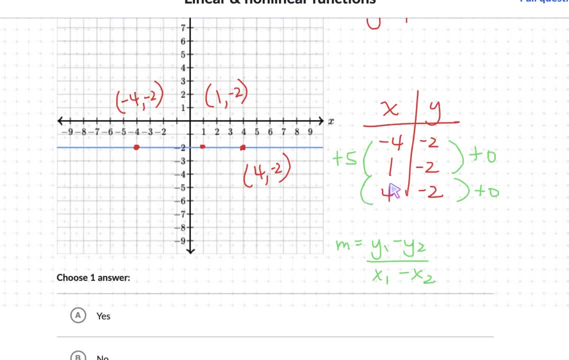 from one to four. I would add three to get there. So here it looks like it's not a constant rate of change, But remember it's the change of y over the change of x. So I have zero over five. that's this number, and this number And that slope is zero. divided by five is zero. 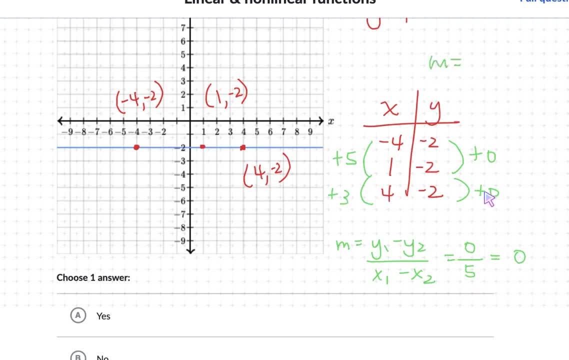 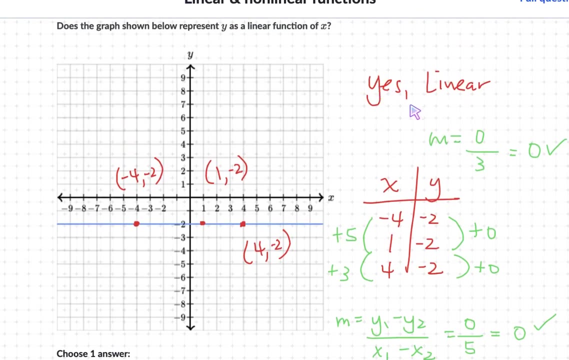 The other slope is 0 over 3.. 0 divided by 3 is also 0. So even though the x differences are not the same, we still get the same answer of 0. It is a constant rate of change. So it is linear because it's a straight line and also, 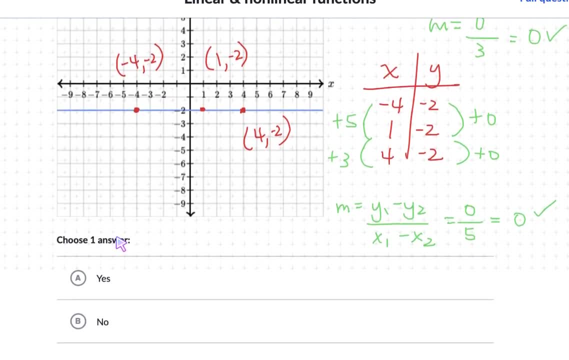 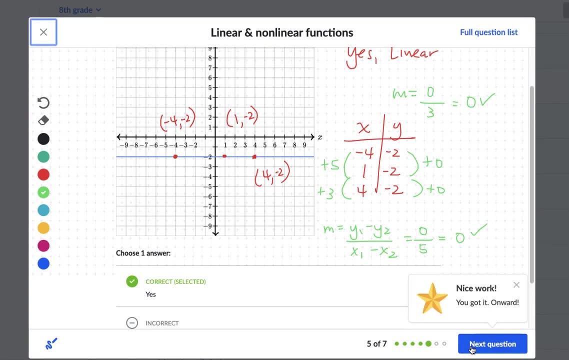 because the slope always comes out to the same number. So is this a linear function? Yes, That's two different ways that we figured out the answer. Again, you don't have to do all this. If you already have the graph, you can just eyeball it. 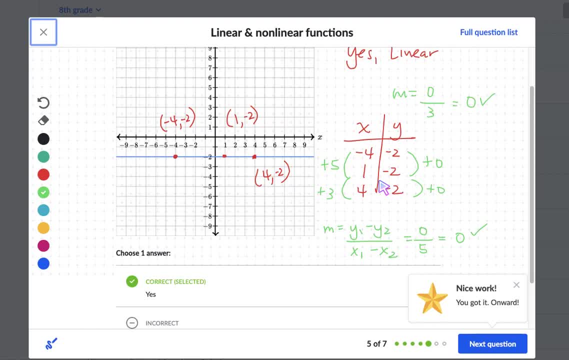 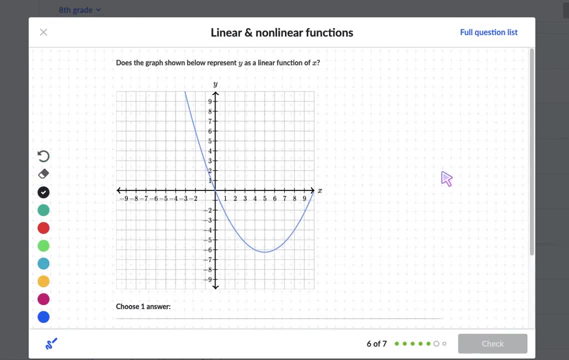 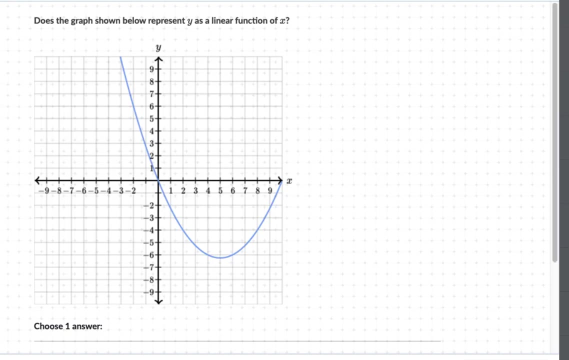 and see that it is a straight line. However, that's how you would create the table of values. Here's another question. Go ahead and pause the video and try on your own. Is this a linear function? All right, I see that this is not a straight line. It. 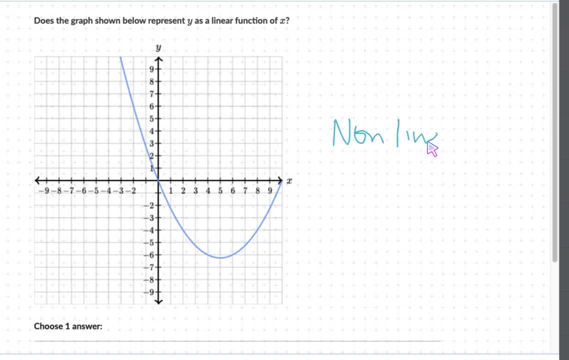 does a little dip, so I'm gonna say that this is non-linear. If I wanted to create a table of values, let me choose some pretty points. That's also a pretty point, and that's also a pretty point. So I have negative 2,, 2, 1, and 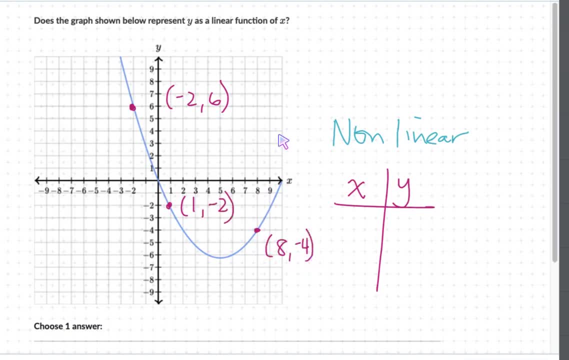 1. then 8, negative 4.. So negative 2, 6, 1, negative 2, 8, negative 4.. And I'm going to calculate the slope, Because later on for my slope I need the change in y over the change in. 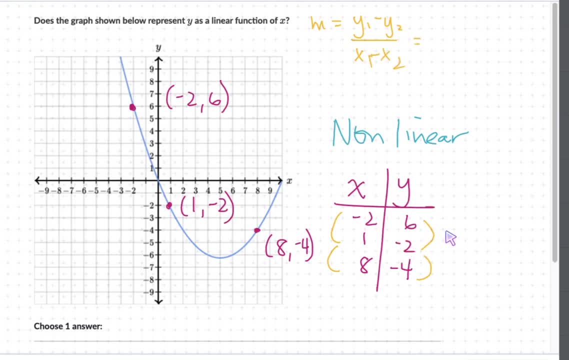 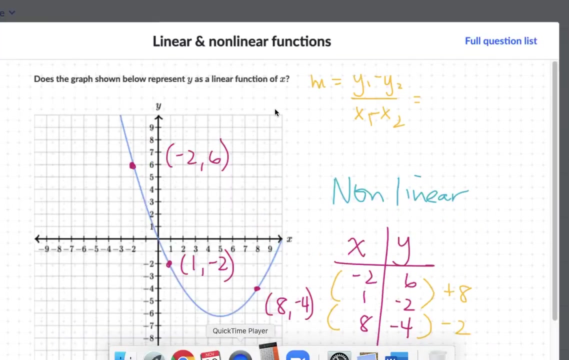 x 6 to get to negative 2, we would have to add 8.. Negative 2 to negative 4, we would subtract 2.. And if you need a reminder on how to do that, you can just use your calculator. 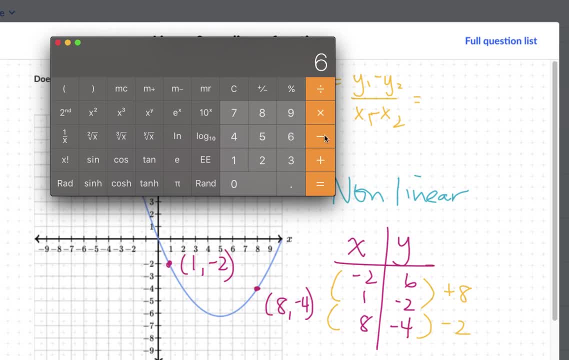 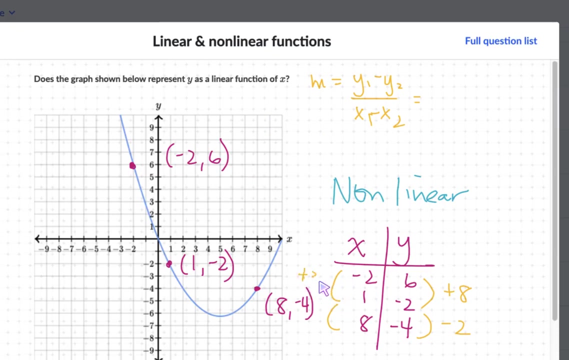 So literally what I can do is I can subtract: So 6 minus negative 2 gets me that 8. And negative 2 minus my negative 4 gets me a 2.. So it is getting smaller, And over here this is going to add 3 to get there 1 minus 8, or 1 to get to 8 is plus 7.. Okay, So then 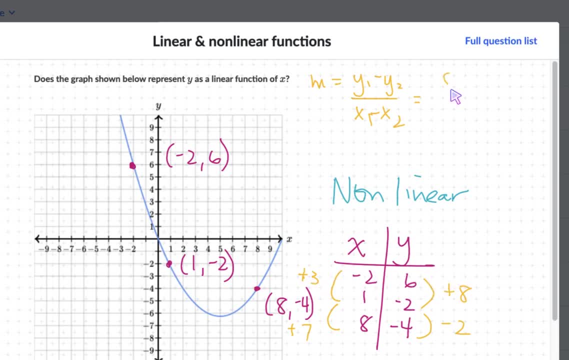 if I were to do the same thing over here, I would subtract the slope. So I would subtract the slope. If I were to calculate the slope, it would be 8 over 3 for one of them And the other slope would be negative, 2 over 7.. Those two are not equal, So further proof. 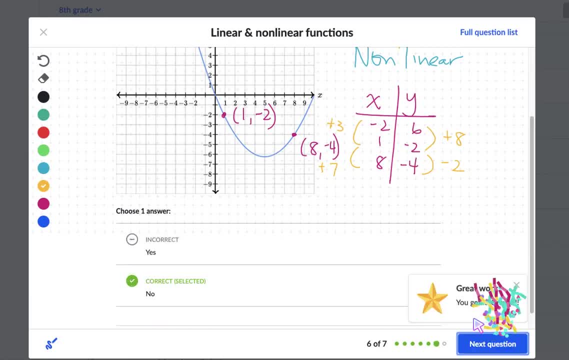 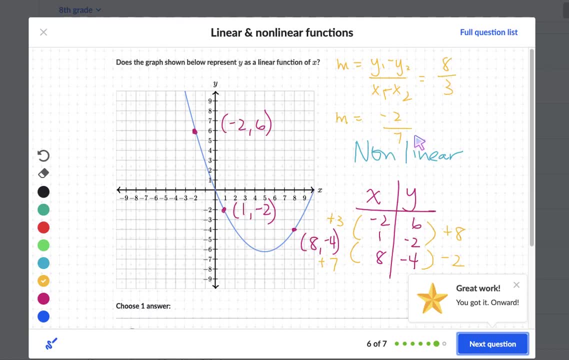 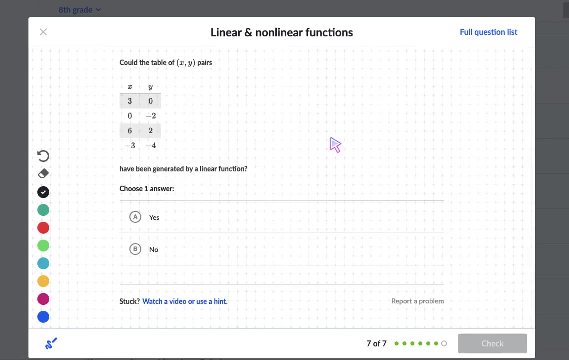 that is nonlinear. So what this slope is showing me is that first it's positive- 8 over 3.. And then it's negative, So it's literally decreasing and then increasing. So it's not constant. Okay, One last question. So here they don't give you the graph, So you're going to have 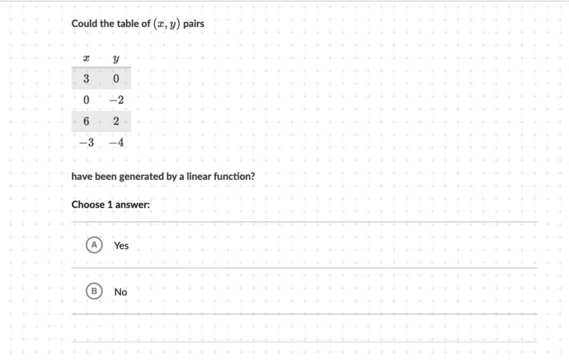 to use the slope that we talked about earlier. Go ahead and pause the video and try this on your own. All right, So just like before, we're going to calculate our changes in x and changes in y, Remember the y differences go on top and the x differences go on the bottom. Let 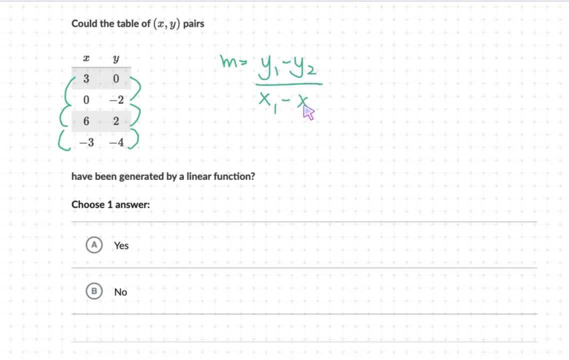 me actually rewrite that, Okay. So again we're subtracting 0 minus negative 2, or to get from 0 to negative 2.. So that's going back two spaces. This is going forward four spaces. So if I had negative, 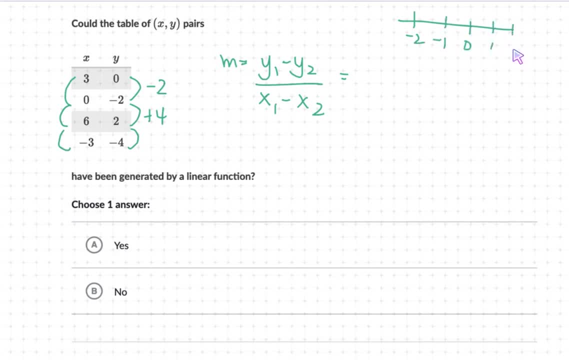 2, it's going forward 1,, 2,, 3,, 4 spaces to get from negative 2 to positive 2.. 2 to negative 4, it's going backwards 4 spaces plus another 2 more, So it's going backwards 6 spaces. 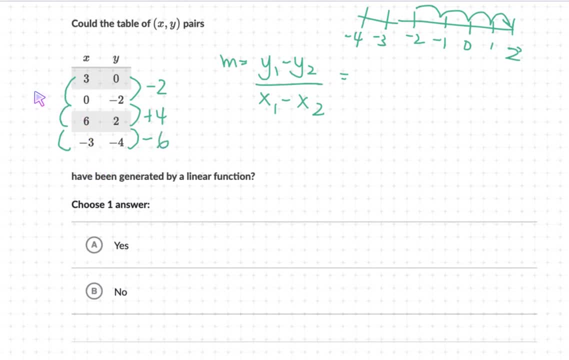 3 minus 1, that's going backwards 3.. This is going forward, 6.. This is going backwards, 9.. Okay, So my slope is my change in y over change of x. I have negative 2 over negative 3 for one of them. 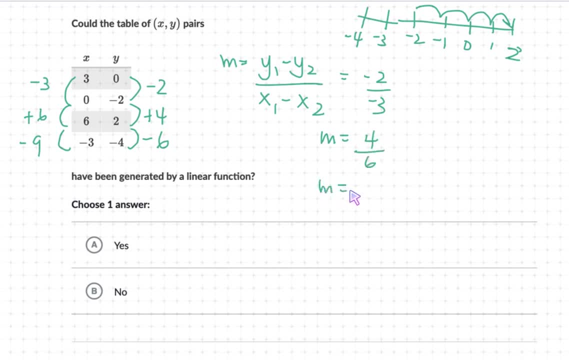 I have positive 4 over 6 for the other, And for the third one I have negative 6 over negative 9.. Now here they look like they're different, but I'm a little tipped off here that something's going on, because I'm seeing a lot of numbers that are divisible. So first, 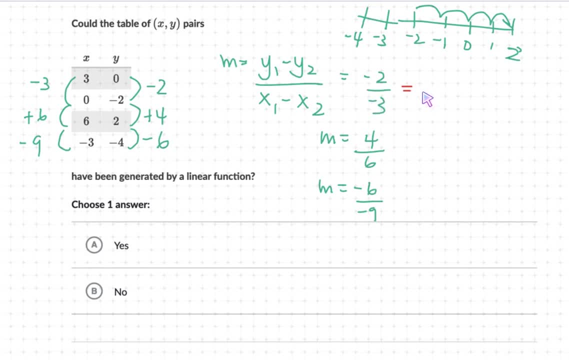 of all, let me—that means I have to simplify Negative 2 over negative 3, I'm going to simplify them to positives, because negatives and negatives cancel out to positive. These are—this is slope, so we need rise over run, So I'm keeping them as fractions Here. I can reduce by 2.. 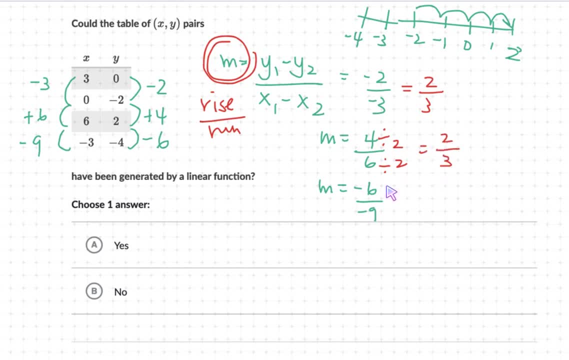 So I get 2 thirds. So far they're actually the same even though they look different. And this one they're all divisible by negative 3. So this would actually be 2 thirds as well. So all the slopes are the same. It means it's actually linear. They're going up at the same.